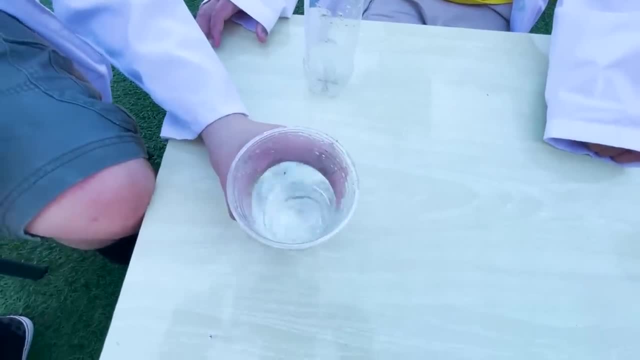 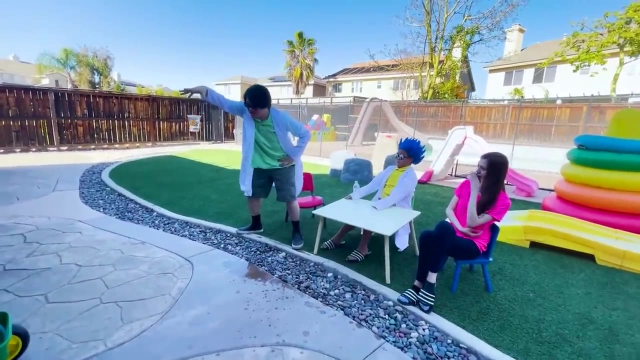 Not so high right Now. you take some water and you shake it a little bit, Then you add your ping pong ball Now back up, because there's a lot of splash going on here. Whoa, Now that's some distance. 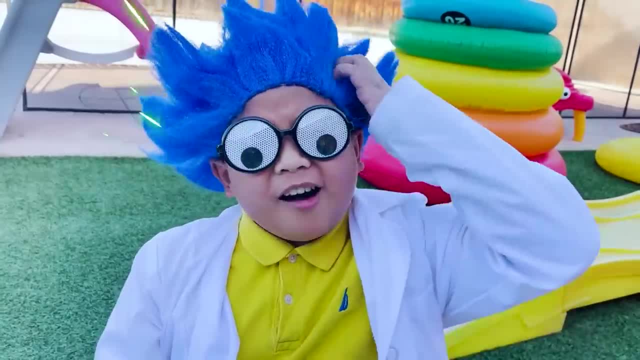 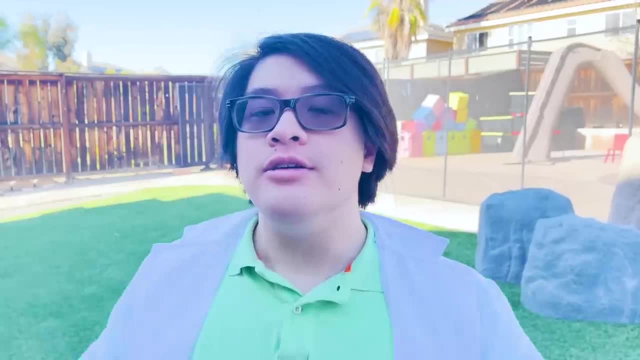 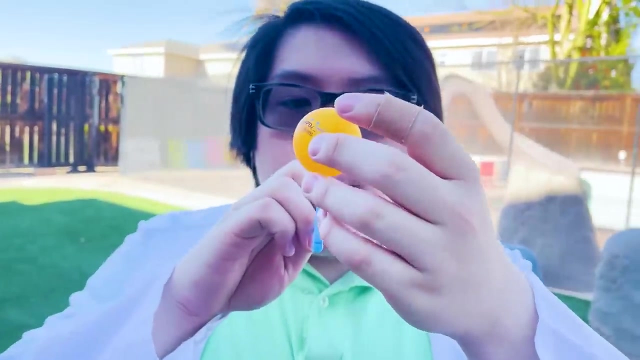 Now let me show you our ping pong ball trick using straws- Straws. How'd you do it? You need to take a deep breath, Then a steady stream of air when you blow out. Let me try, Uncle, Go ahead. 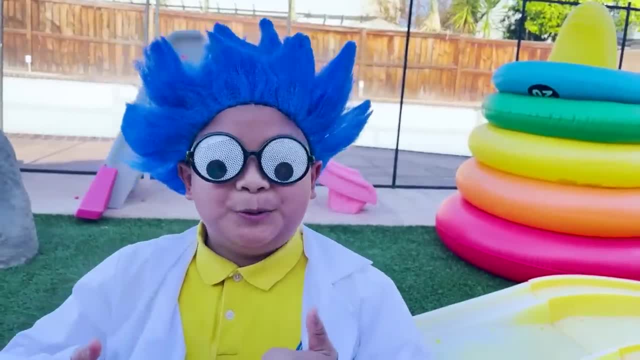 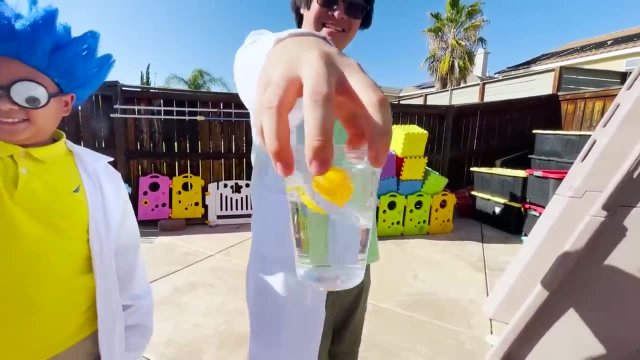 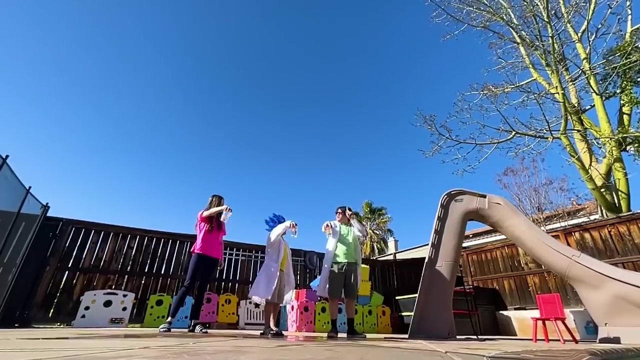 You helped me a lot today, scientists, I learned a lot too. Now let's do a competition. All right, Whoever's ball goes the highest, wins You ready. Three, two, one stop, Stop. Congratulations, Uncle. 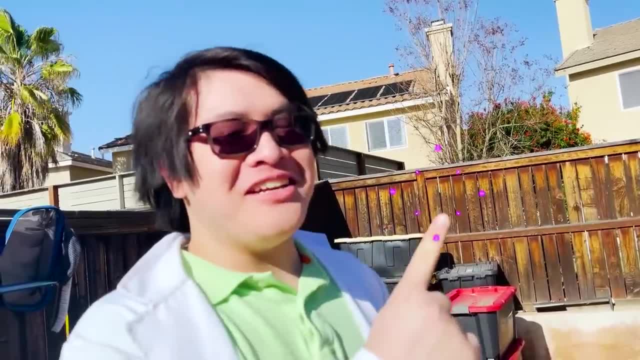 You won, Yeah, Now remember guys, patience is the key. If you fail, try, try again. Wow, This is so cool, Ah, Whoa, Ooh so cool. Another one: Yellow, green and pink. 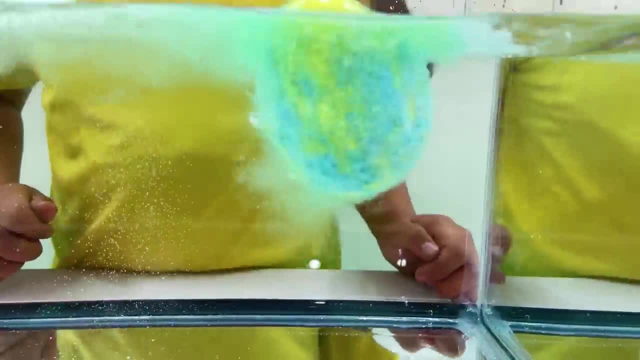 Look at all those colors. Wow, Huh, Jenny, what are you doing? Auntie, look, it's really cool. Ew, Jenny, this wasn't for playing, It's for playing. You can't play, You can't play. 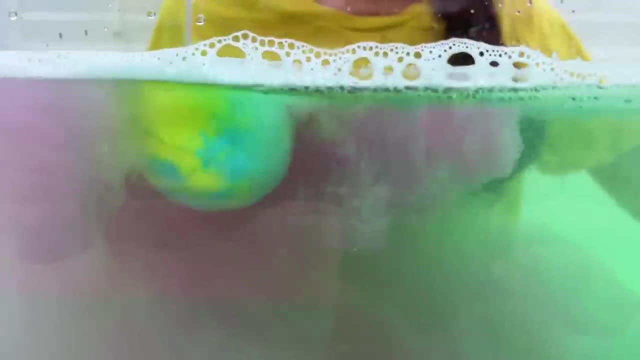 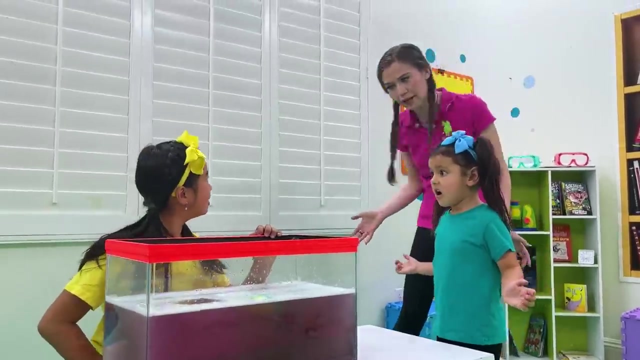 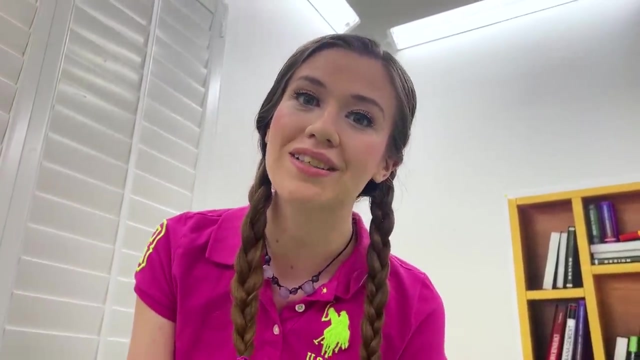 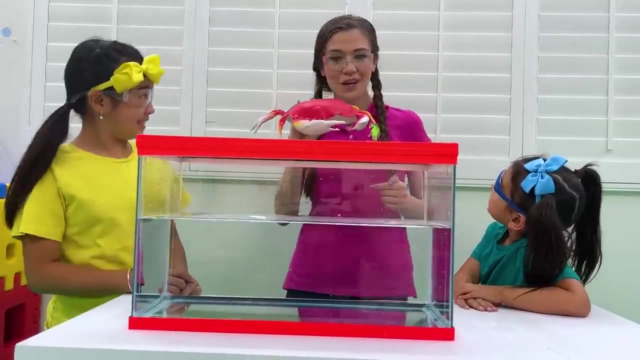 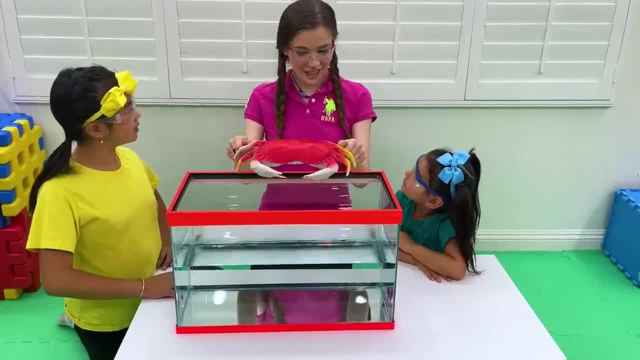 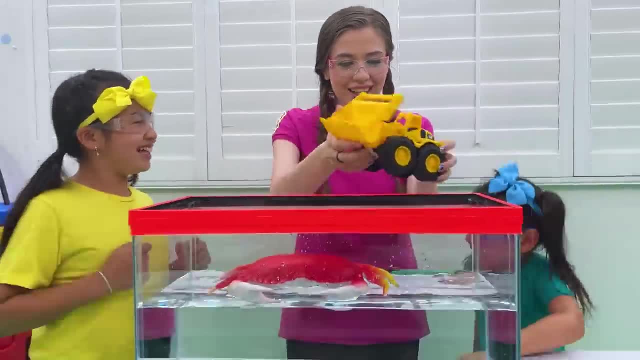 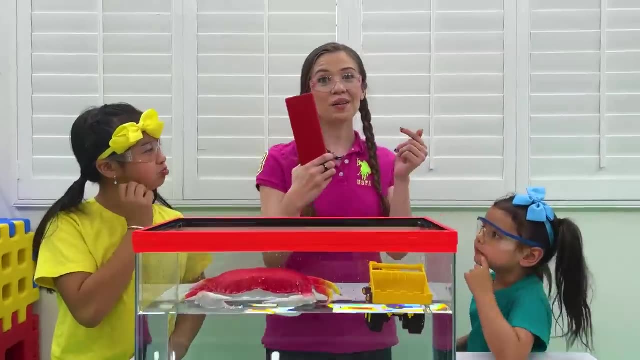 It's floating. What do you think, guys? Float or sink, Sink, sink, sink, sink. Wow, Huh, That's impossible. How about this rock? Is it gonna float or sink? It's pretty big. I think it's gonna sink. 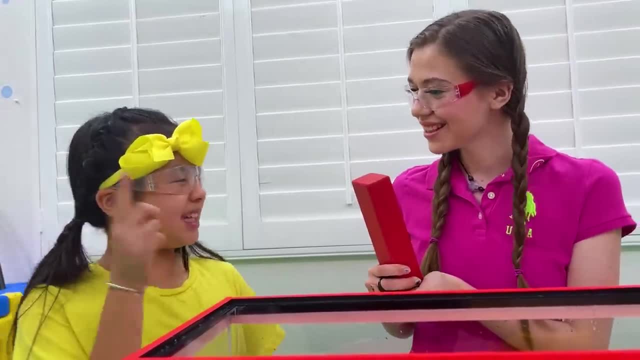 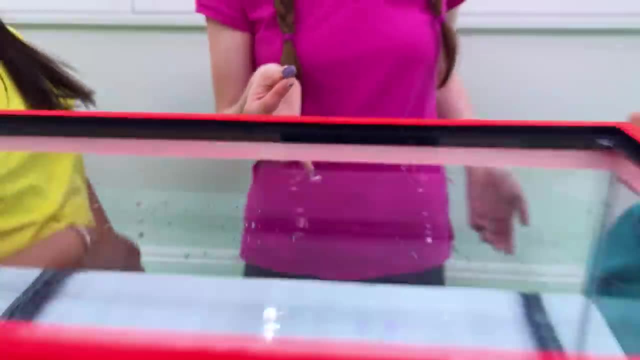 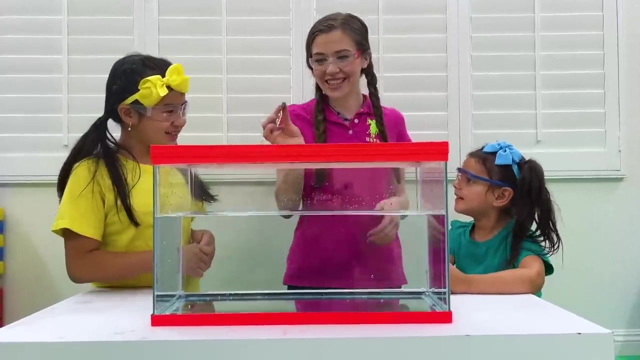 Let's see. Huh, It floated. How about this bath drop? will it float or sink, Sink, float, Float, Float. Go get it. Wow, Float, float, float, float, float. Okay, let's see. 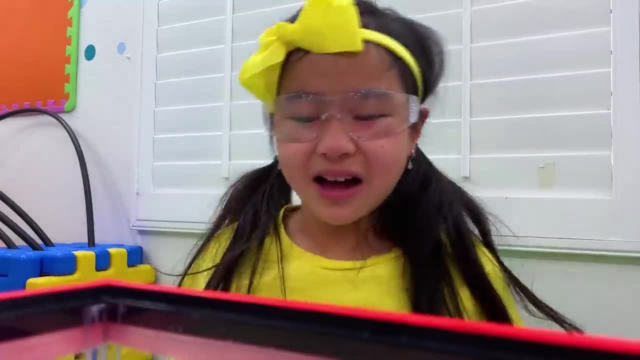 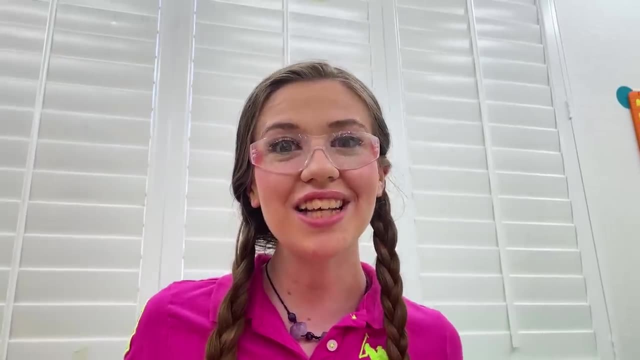 Hmm, let's see. Huh, The bath drop sank. I was lucky. What makes things float or sink, Auntie? It's because of the density of the material. If the material is more dense than the water, it will sink. 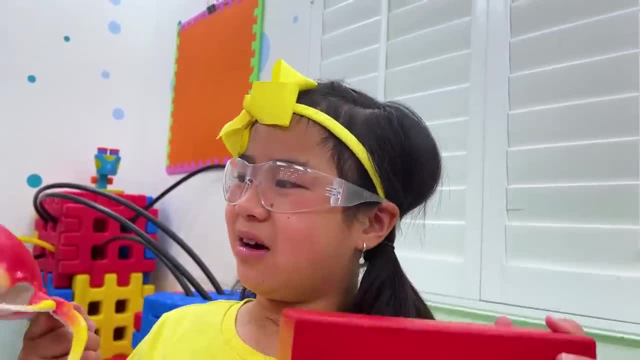 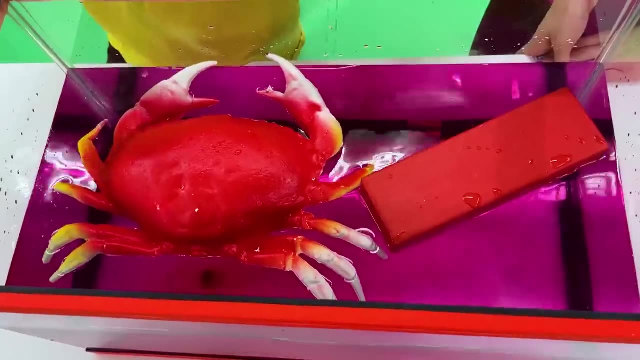 If it's less dense, it'll float. Wow, nice, I thought the size mattered. If it's big it will sink, But if it's small it will not sink. But I was wrong. Both the crab and the block are big, but they float. 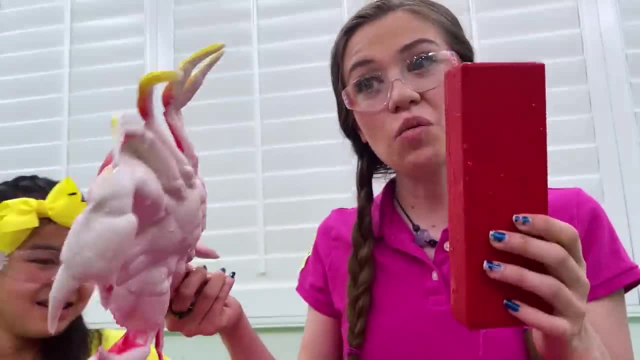 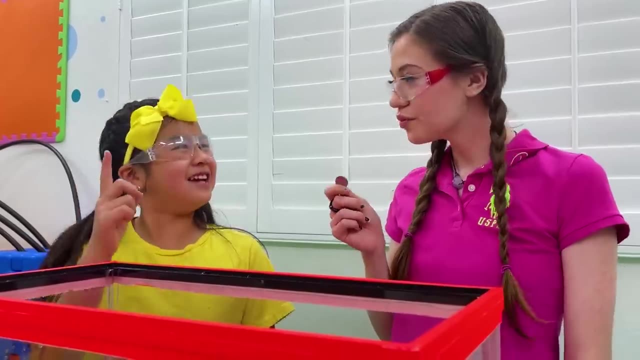 Yes, that's correct. That's because their material is less dense than water, causing them to float. What do you guys think Will the coin floater sink, Float, float? Hmm, are you sure? Maybe sink. All right, let's see. 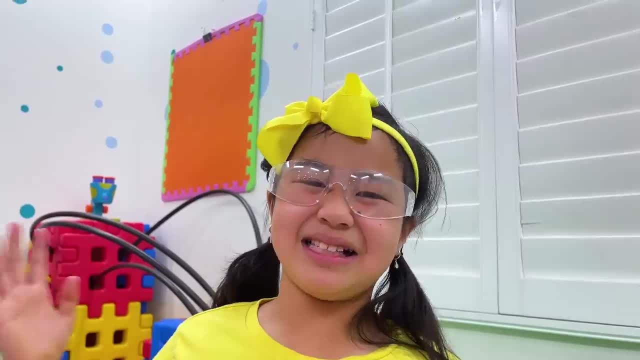 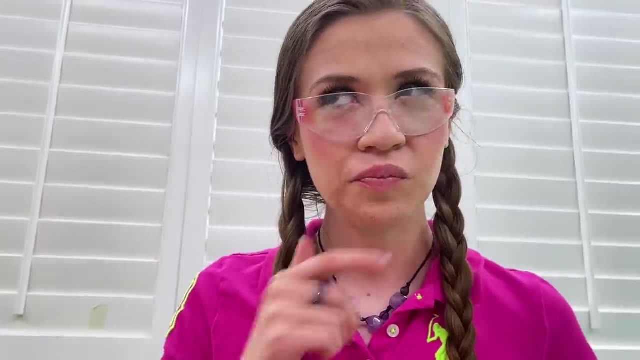 It's C. Finally I got something correct. If you get it right, you'll get a new toy. If you don't, you've got to clean the house for a whole week. Hmm, I think it's going to float. 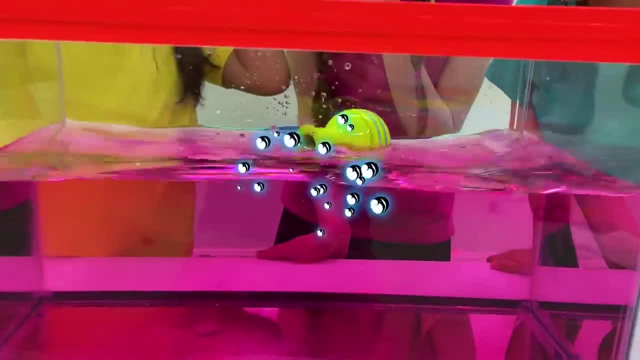 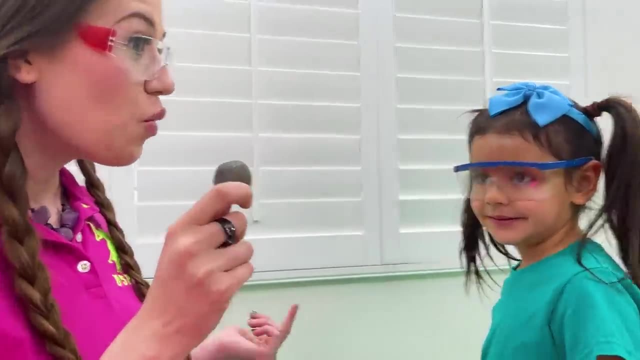 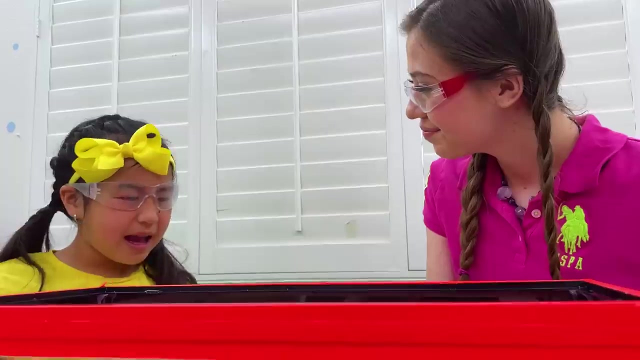 All right, let's check it out, Okay, Huh, No, Uh, clean the house for a week. All right, Ellie, how about this rock? Will it sink or float Sink? We'll see. Auntie, why did the rocking coin sink? 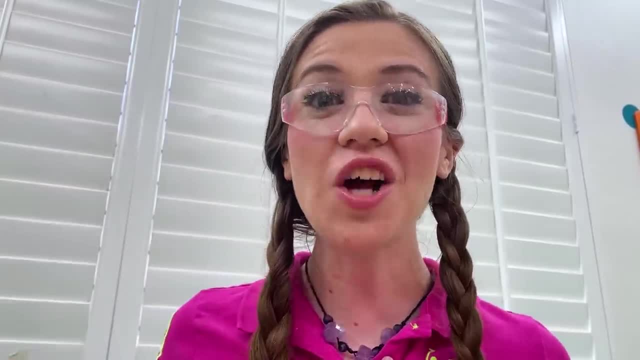 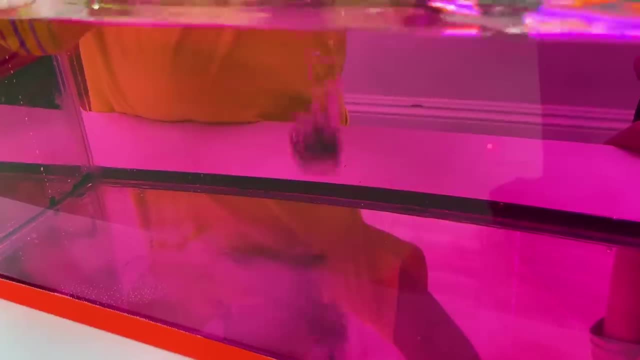 It's so small, Remember, Danny? Size doesn't matter, It's all about the density. Oh, I get it now. The material of the rock in the coin is more dense than water. It made them sink, That's right, Danny. 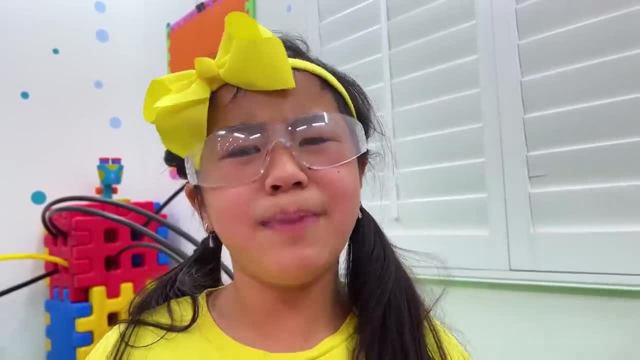 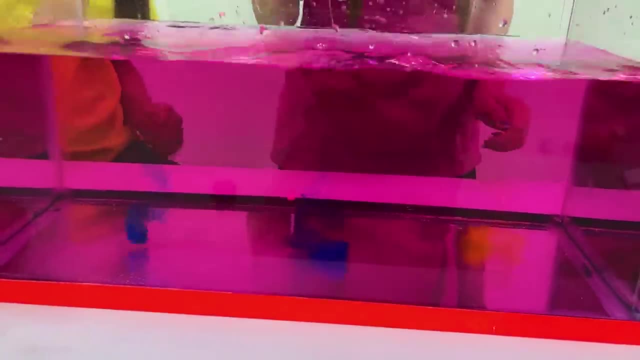 Good job. Thank you, Auntie. I learned a lot today, But I have to clean the house now. Not so fast, Danny, Let's play with more bathrobes. Yay, Yay, Wow, It looks so colorful. 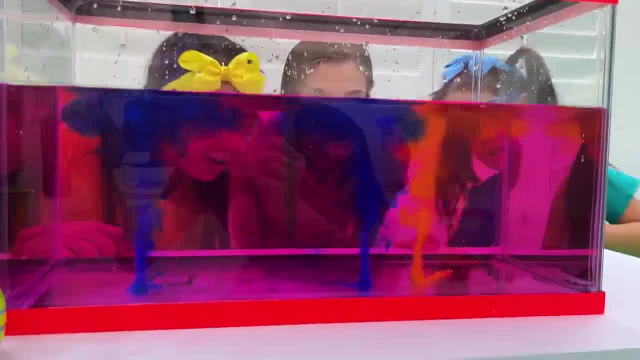 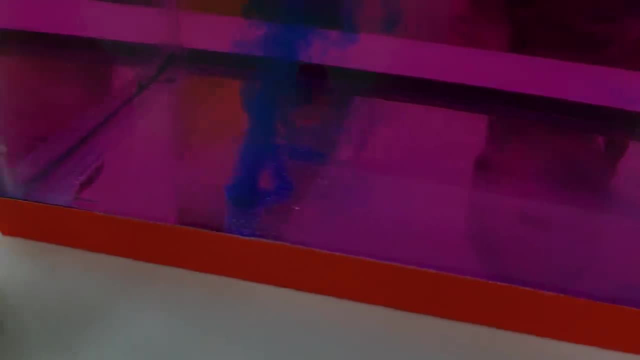 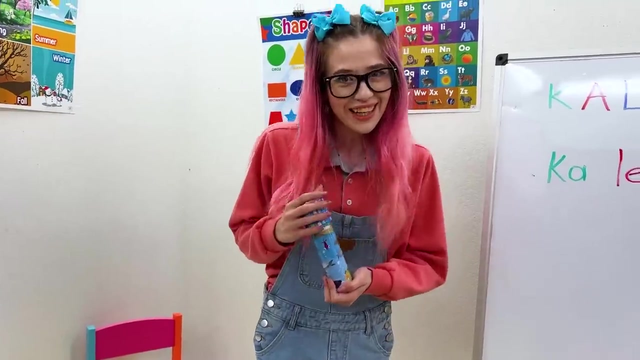 Wow, Blue, blue, yellow. Wow, look at the yellow, It's a bubble truck. Wow, Wow, Kaleidoscope. Not exactly. How about you, Danny, Kaleidoscope? Good job, Danny, Here's your kaleidoscope. 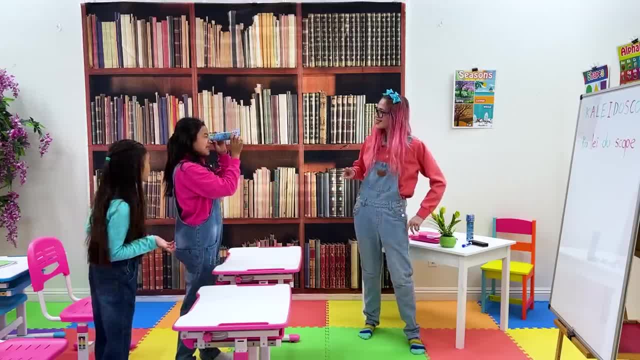 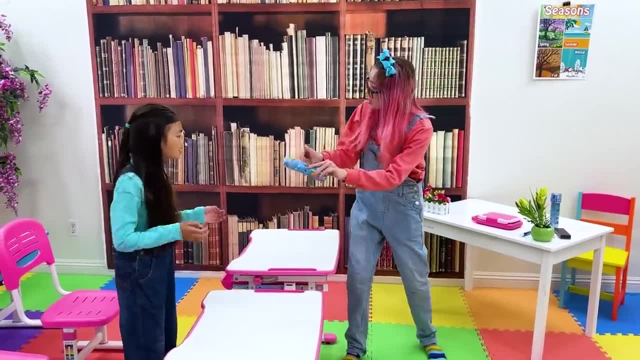 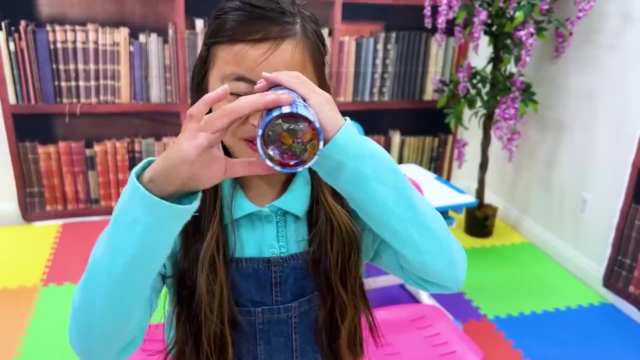 Now pronounce it three times: Kaleidoscope, kaleidoscope, kaleidoscope. Oh, where'd Danny go? Wow, this is cool. Wow, look Danny's inside. Whoa, Whoa, Whoa. Kaleidoscope, kaleidoscope, kaleidoscope. 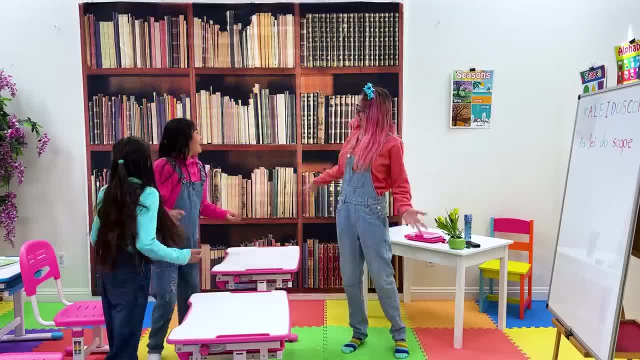 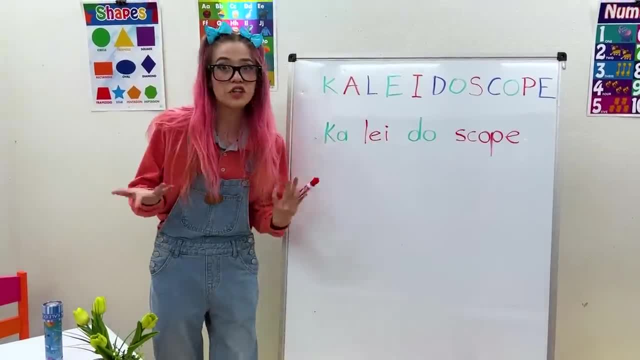 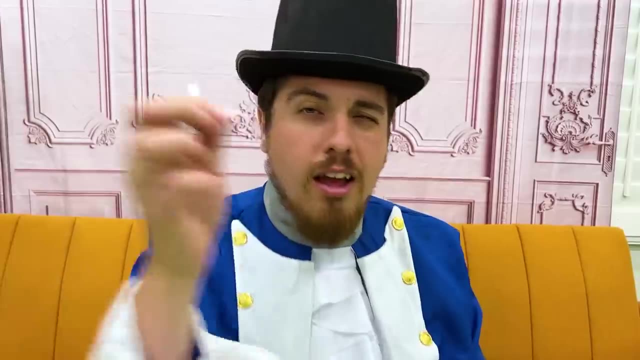 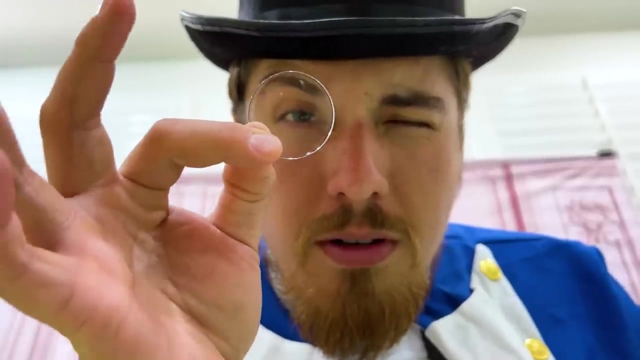 Uh, wrong pronunciation. Ah, Charlotte, you can do it. Let's try again. Kaleidoscope- Kaleidoscope means to watch beautiful shapes. Kaleidoscope- Wow, Yeah, very handsome today. Oh, those colors are beautiful. 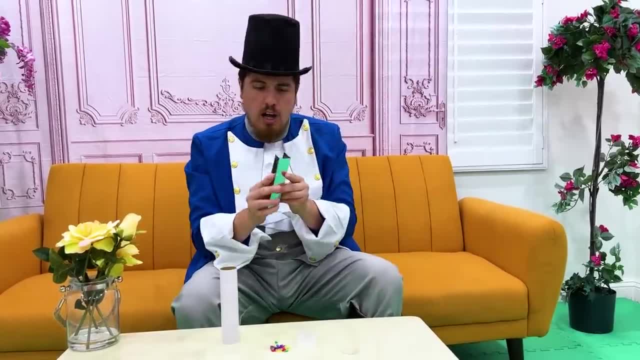 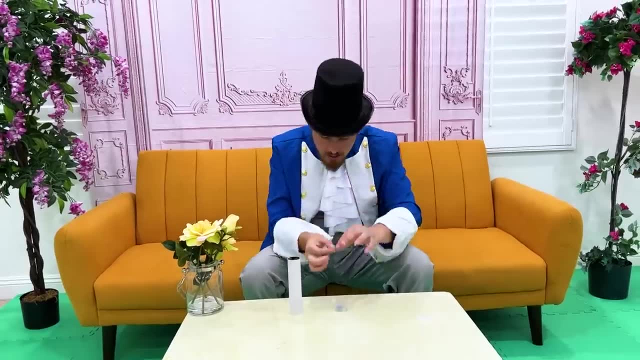 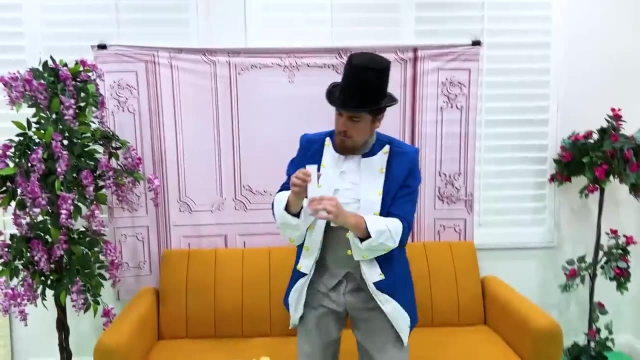 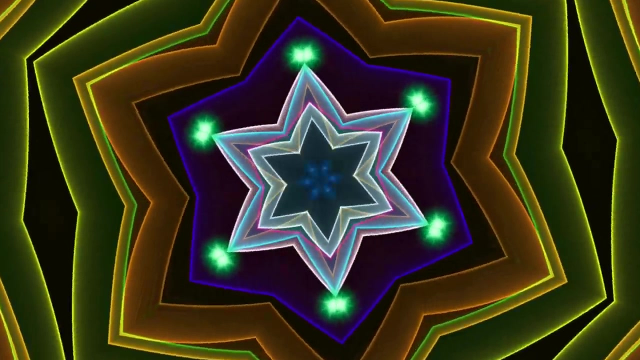 Hmm, we're going to need a tube. Hmm, let's put the mirror inside. Ah, I can put the colored tiles in here. My lens, Awesome. And for the final part, Wow, these images are beautiful. I'll name it the kaleidoscope. 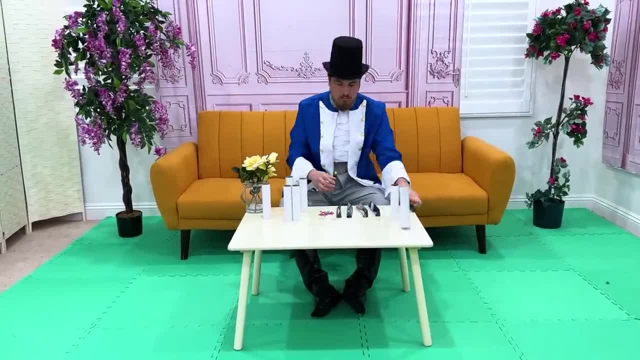 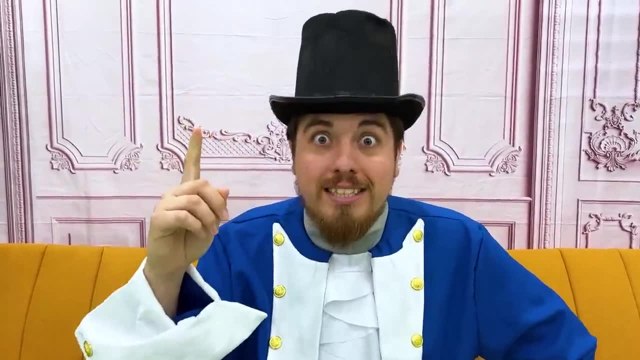 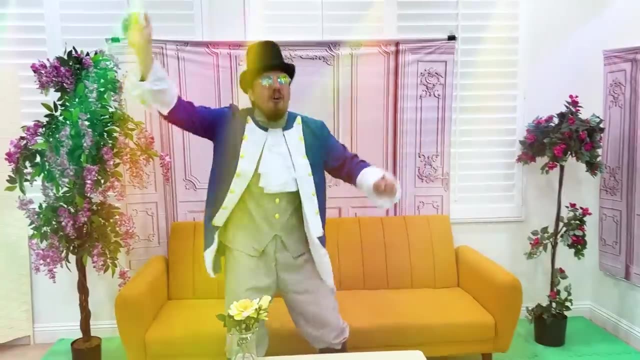 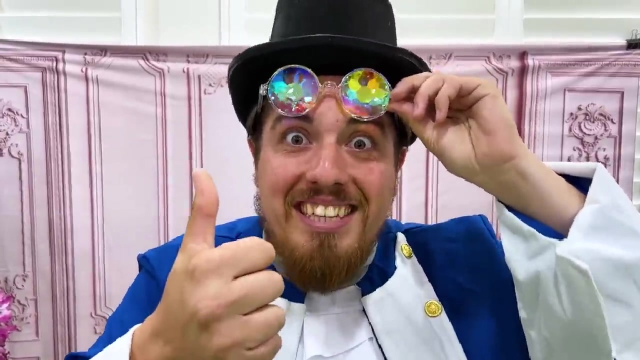 Kids are going to love it. Ah, I can also make kaleidoscope glasses. Oh yes, Whoa Cool, Let's sell these kaleidoscopes in glasses. He sold many kaleidoscopes. Wow, Nice Oh. 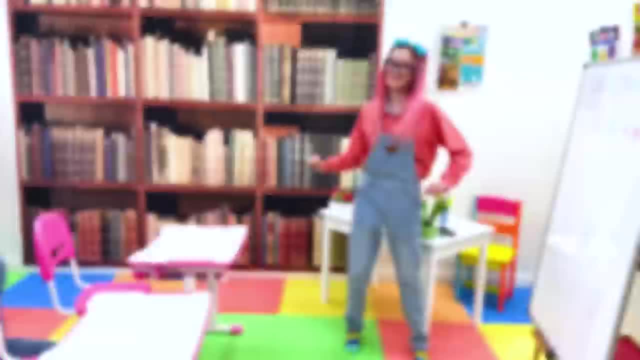 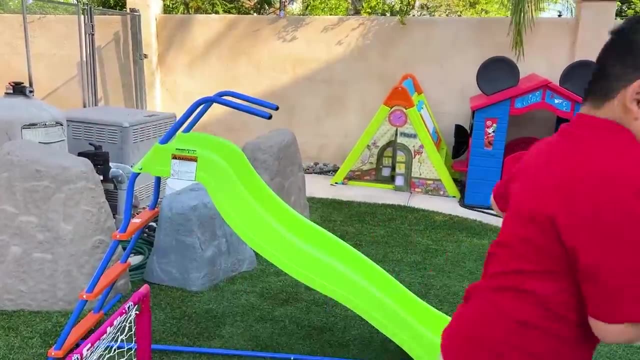 Looks like class is over. Bye kids, Bye Bye, Lyndon. Lyndon, Danny has a kaleidoscope. Kaleido-what? Never mind, Never mind, Just follow me. Wow, This is so cool. I'm hungry. 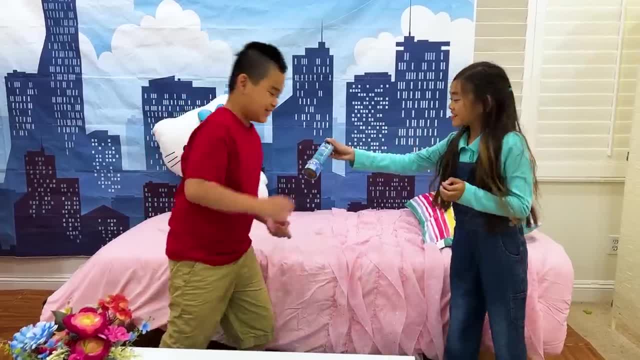 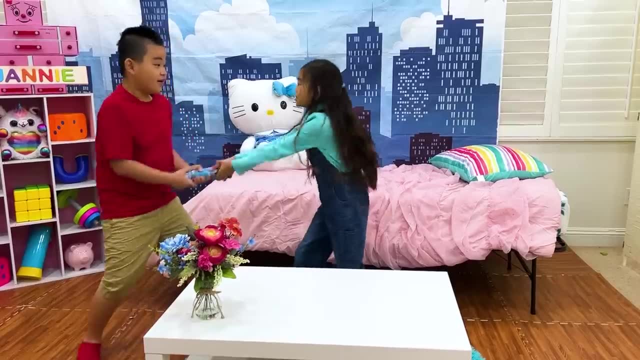 It's the kaleidos. Whatever, Lyndon, check it out. Wow, Let me use it. No, No, Let me use it. I want to watch more. No, No, No, No, Oh, no, Uh-oh. 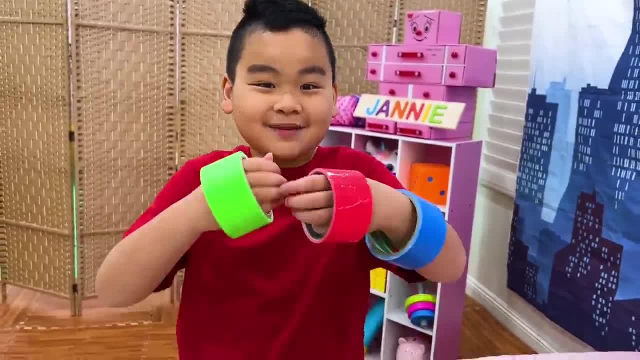 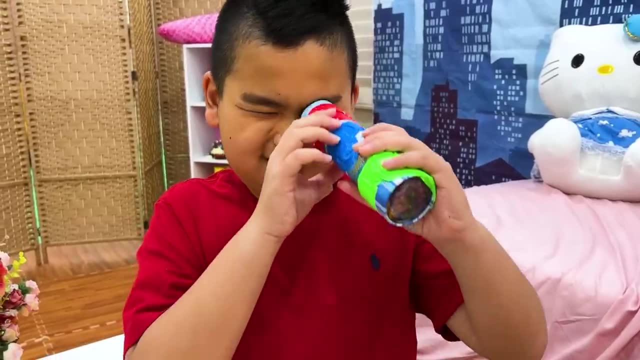 It's broken. Uh-oh, I don't think it's working. Let's fix it with tape. Good idea: The last tape. Let's try it. Uh-oh, What happened? Let me see. Uh-oh, It looks like it's not working. 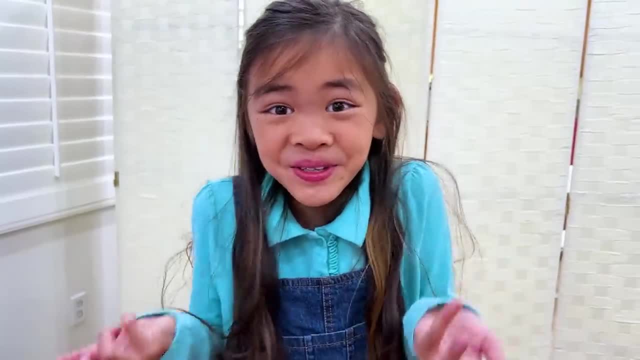 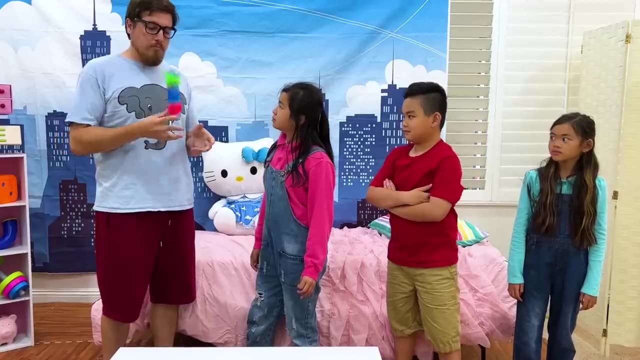 Huh, My kaleidoscope. Sorry, Danny, We broke it. Oh Danny, why are you sad? My kaleidoscope is broken. Hmm, Let me see. Hmm, I can get another one for you, Okay, Hi. 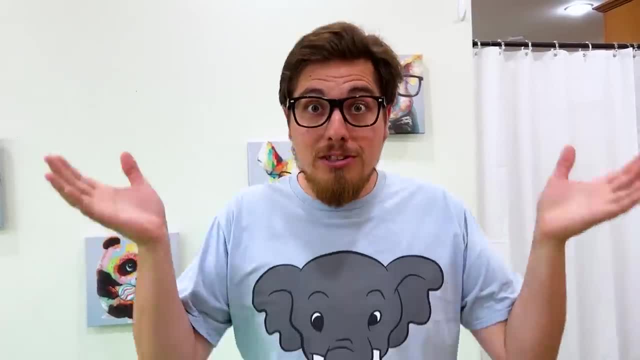 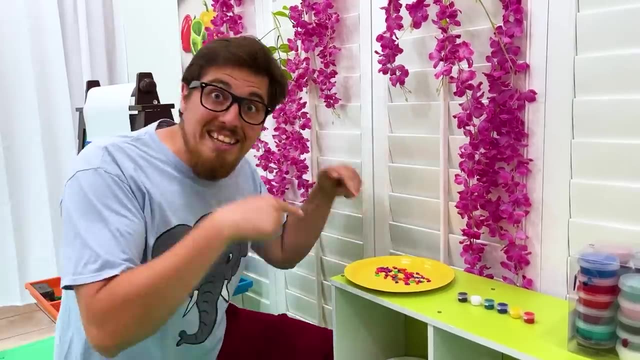 Hi, I'm looking for materials to do crafting. Go ahead, Go ahead. You're in the right place, All right, Thank you. Hmm, Ah, I need these. Yeah, Also these tubes and these lenses. Do you have mirrors? 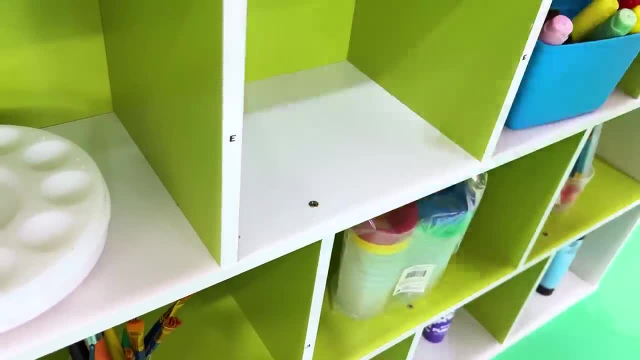 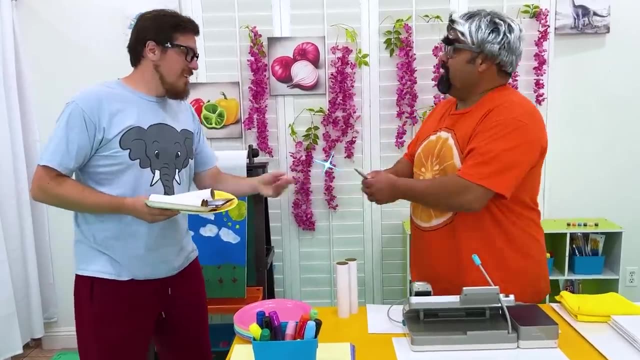 Oh, but of course, Let me get them for you. Here you go, Thank you, I'll take all these $24.99.. Here you go, Thank you. Bye, Bye. Let's make kaleidoscopes, Let's bend these mirrors. 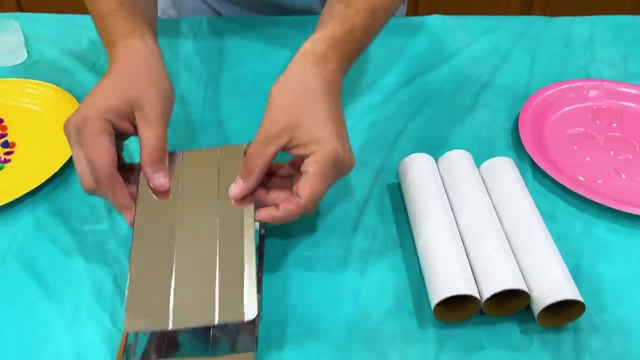 Then we can put the colorful tiles into here- Awesome- And then put the lens on. Now we can connect them together, Wow. And attach a little eyepiece- Wow, Beautiful. The kids are going to love it Yay. 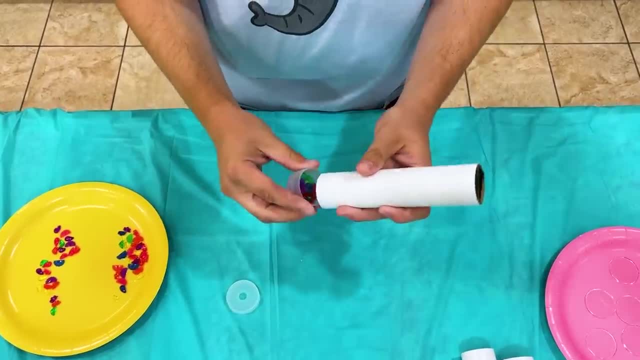 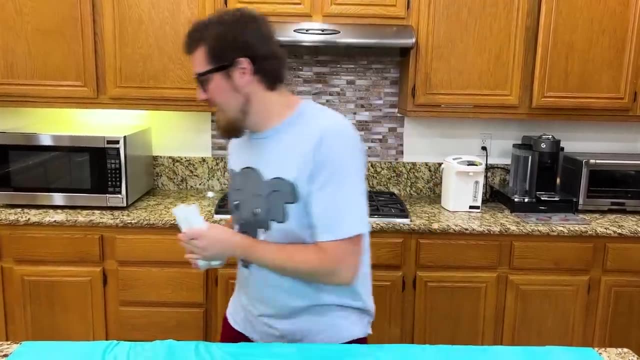 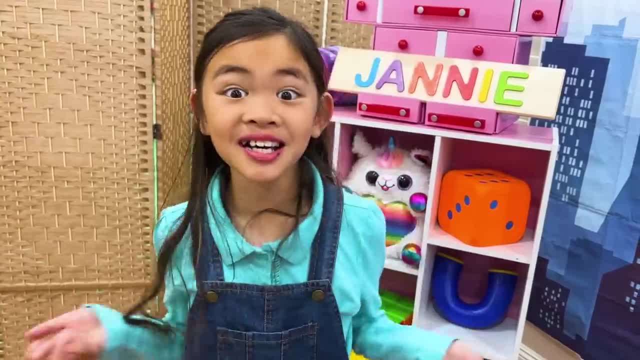 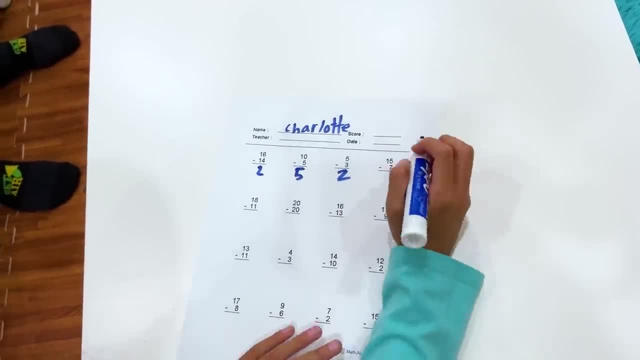 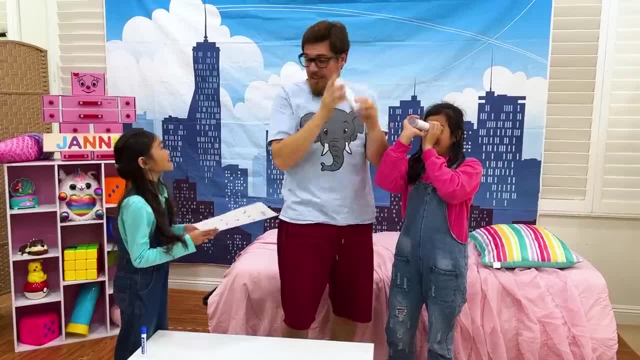 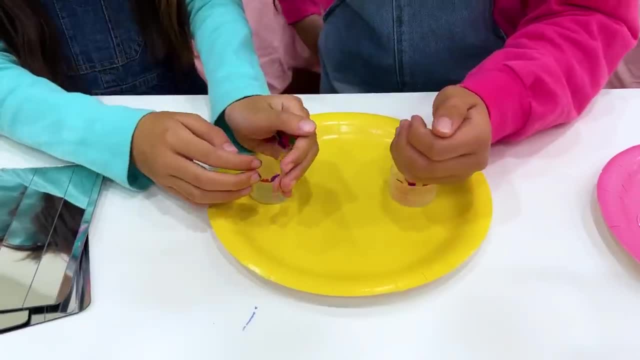 Eight seven. Uncle Zapp, I'm done with homework. Let me see. Ah, Very good, Now you can play. Then we can make more kaleidoscopes. Yay, Let's put the mirror. Yes, Ready. 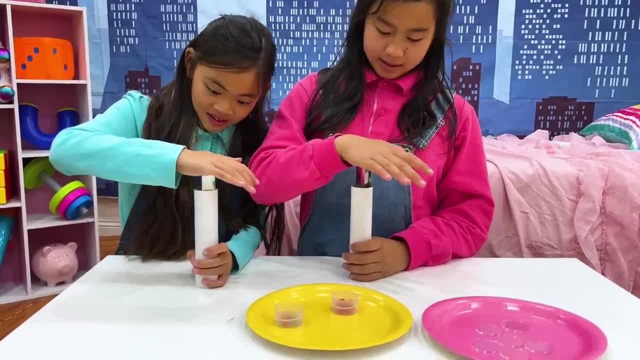 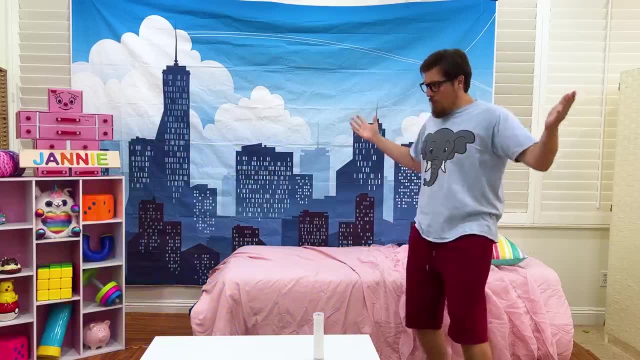 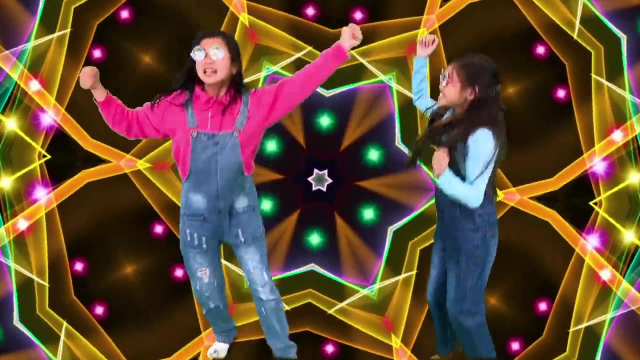 Let's put the mirror on: Wow, Oh, wow, There we go. I love it. Wow, Colossus. Huh, Where'd they go? Ah, there they are. Wow, Don't do it, I have no choice. 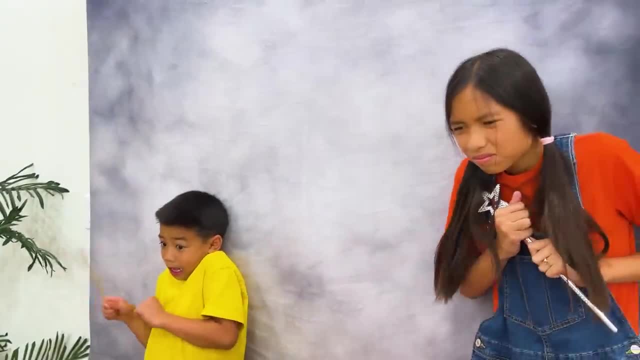 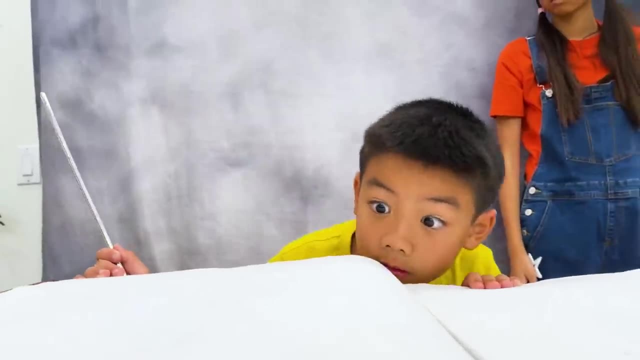 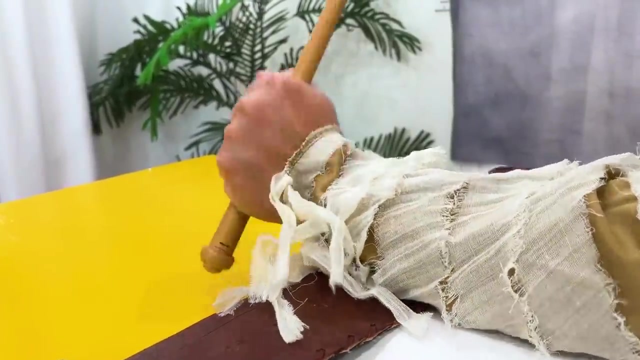 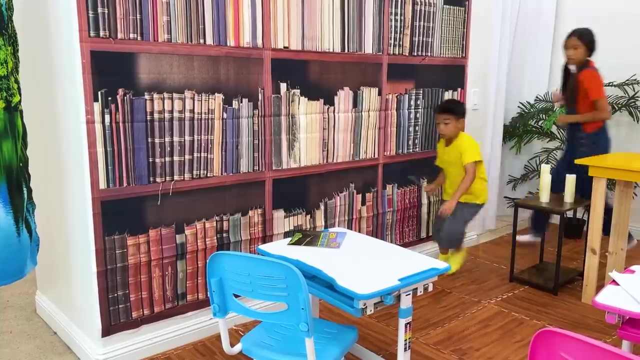 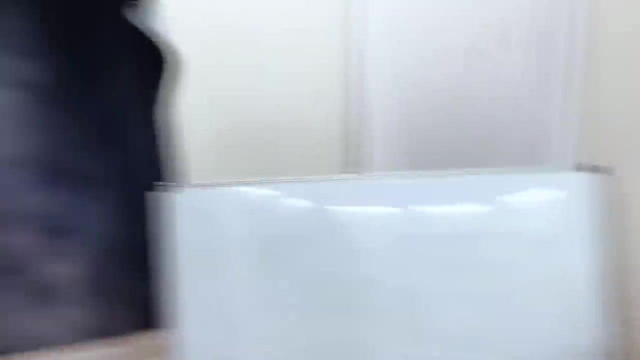 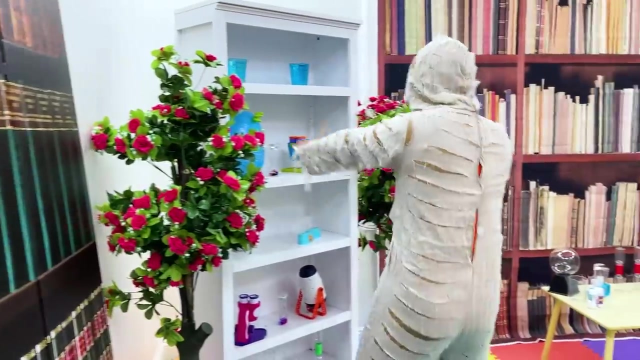 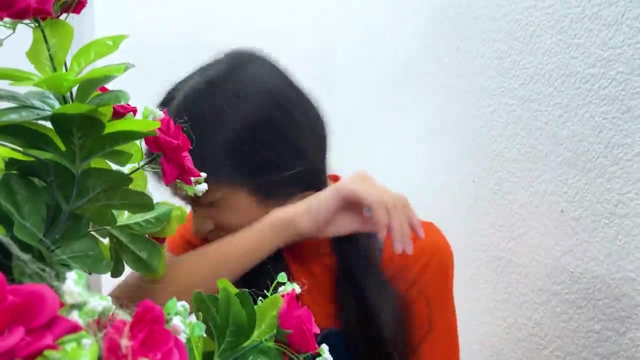 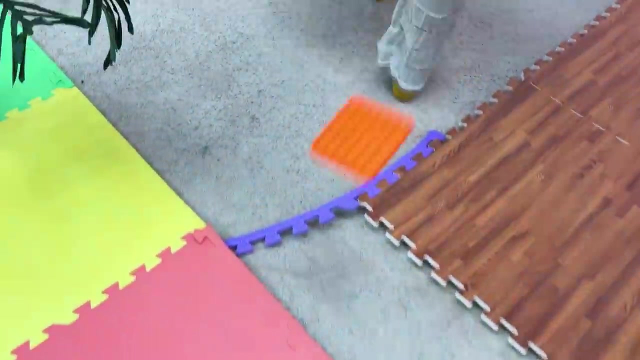 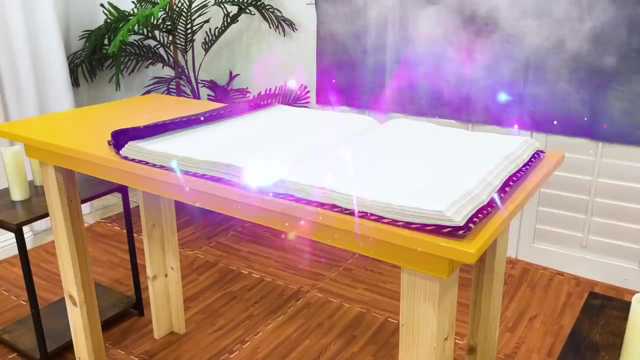 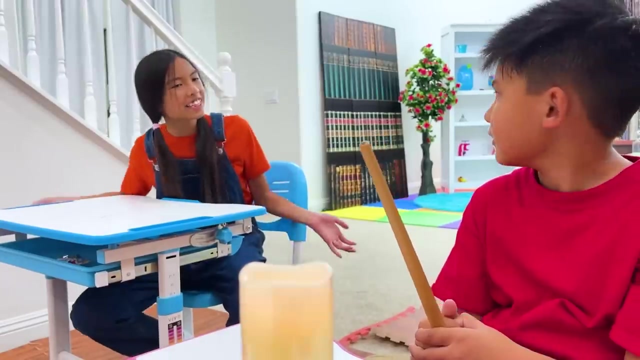 Wow, It's working. Oh, stop, Whoa, What is it doing? Hey, what's going on here And why is my book open? Well, the thing is Ta-da. Wow, Way to go, Leo, You're so talented Leo. 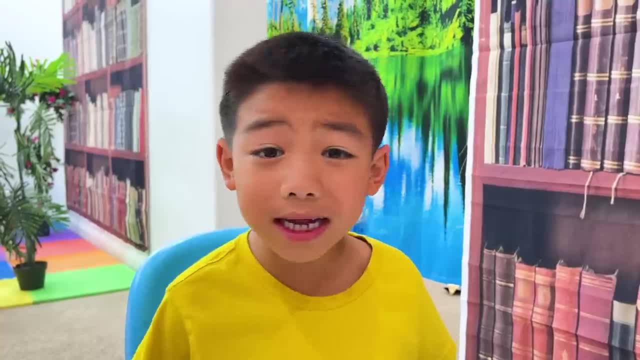 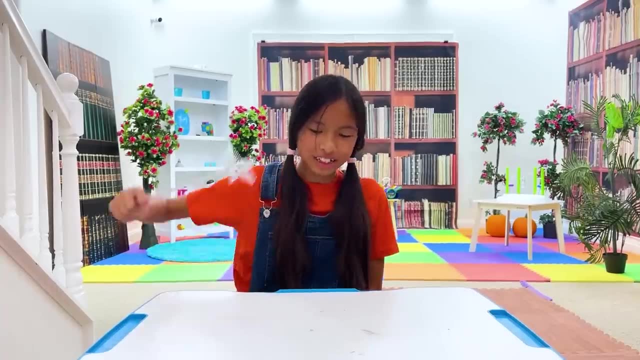 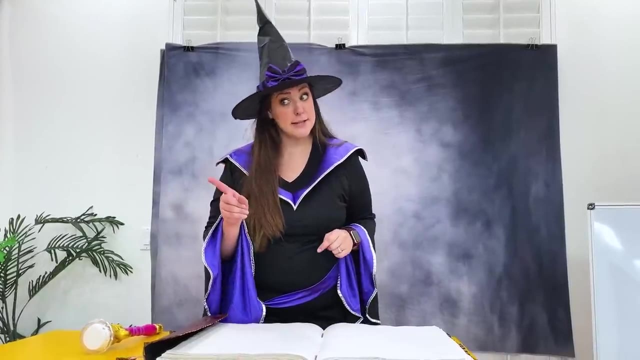 Thank you, Wendy. Whoa, Wow, it disappeared. Where did it go? Genius, Genius. Well, I want to try. I want to try too. Okay, class Tomorrow, there's a test. Make sure you study as hard as Liam. 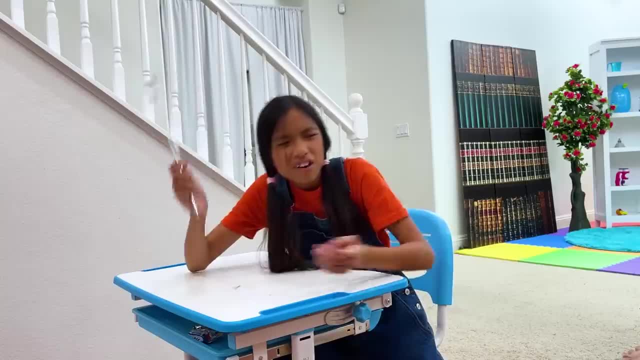 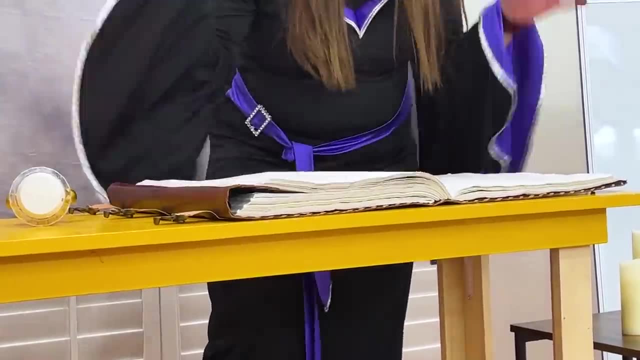 What? There's a test. Yes, I love tests. How are you so excited for a test? Hey, Wendy. What is it, Eric? There may be a spell in that book to make us as talented as Liam. You think so. 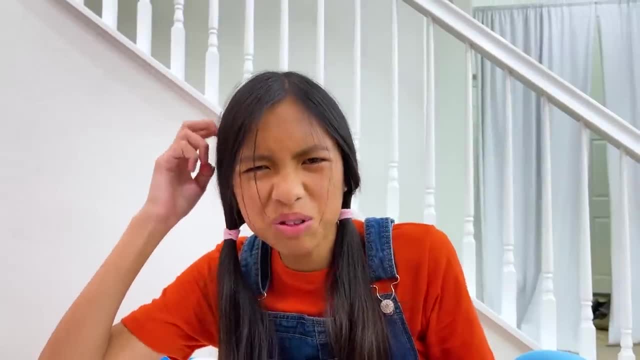 It has to be. It's the teacher's book. I don't think that's possible. I think we should just study. I guess you're right. All right, It's recess time. Yay, Why are you not getting up, Eric? 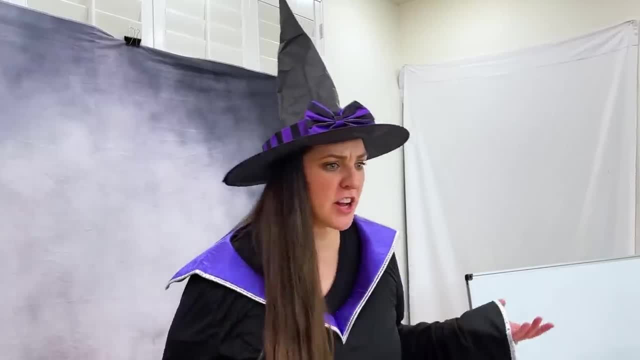 Yeah, Eric, Why are you not getting up? It's recess time. I'm going to start on my studies early. Wow, Okay, That's really great, Good discipline. Oh yeah, I'm going to start on my studies too. 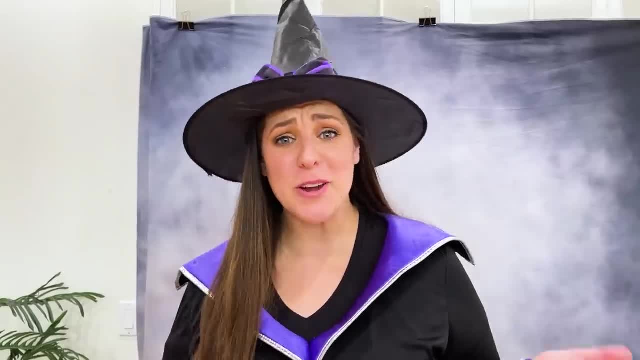 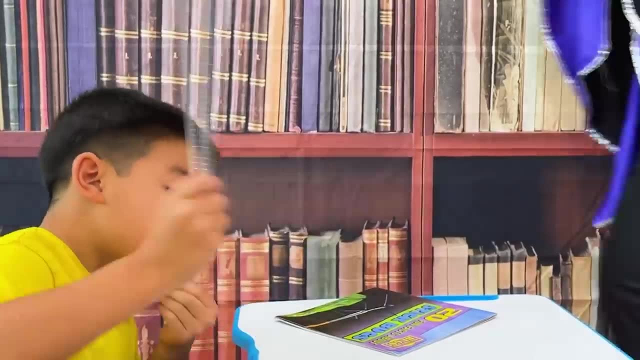 Wow, I'm really proud of your guys' dedication to your study. Yeah, Okay, You start studying. I'll see you guys later. You ready, Wendy? You've got to be very, very careful. Careful is my middle name. 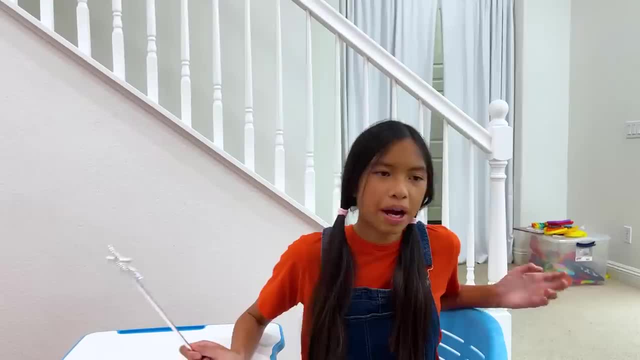 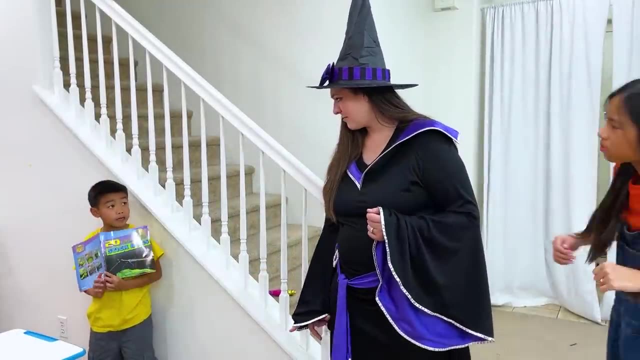 Right, Ooh, Right there. Wait, Is that the spell? I'm sure? Sorry, I just want to be as good as Liam, Me too. We have no time for apologies. We have to find what you let out back here. 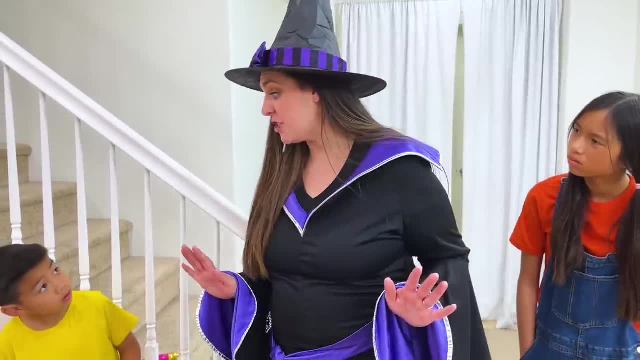 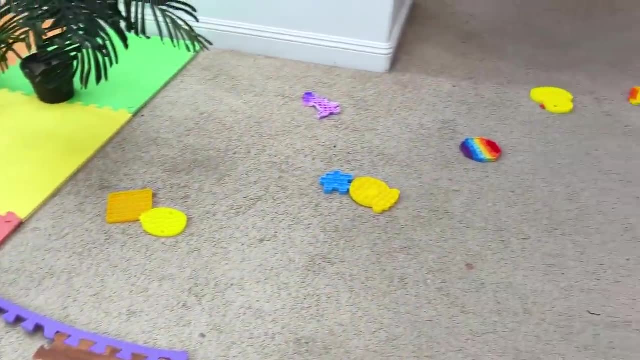 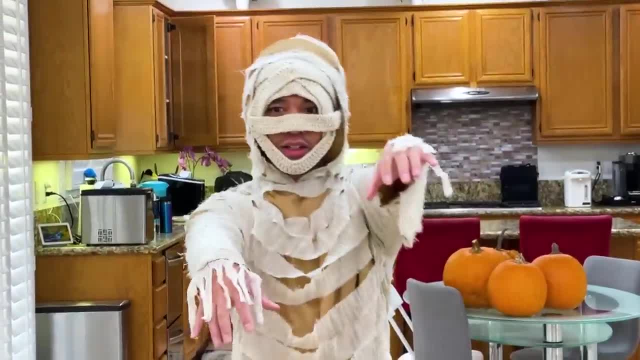 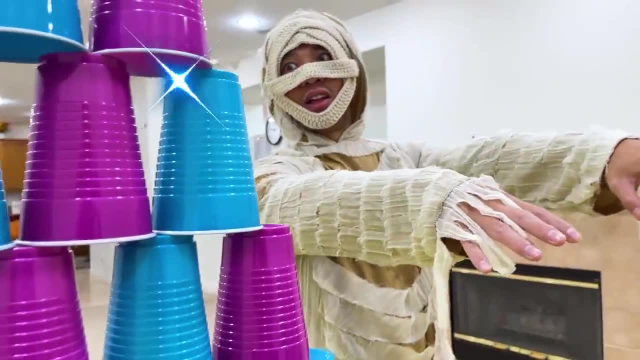 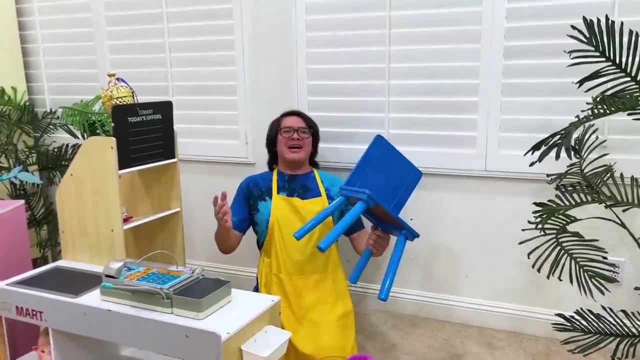 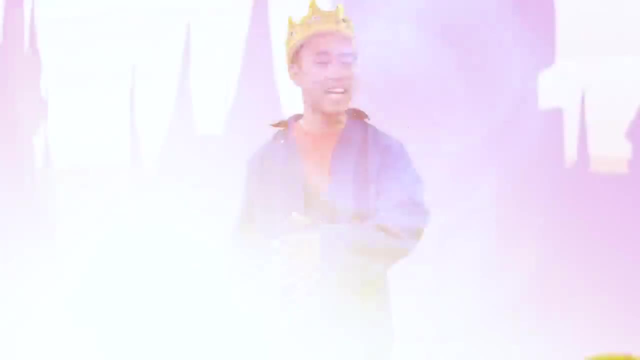 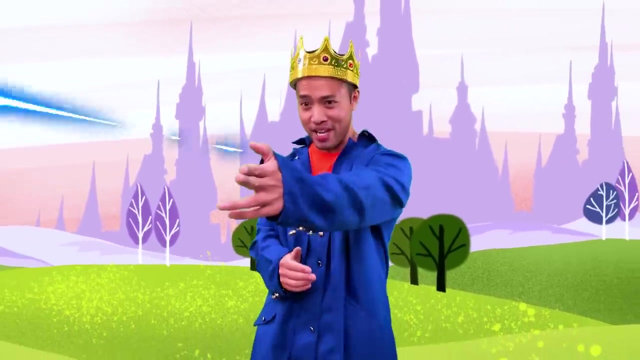 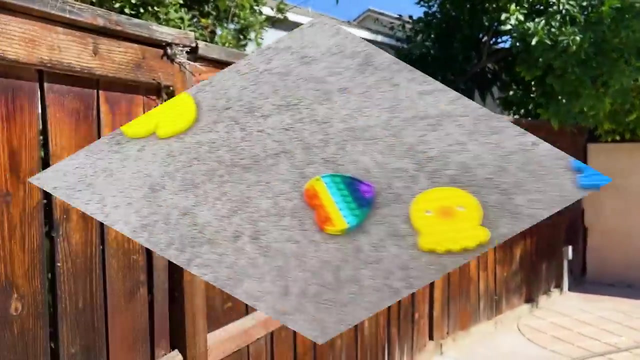 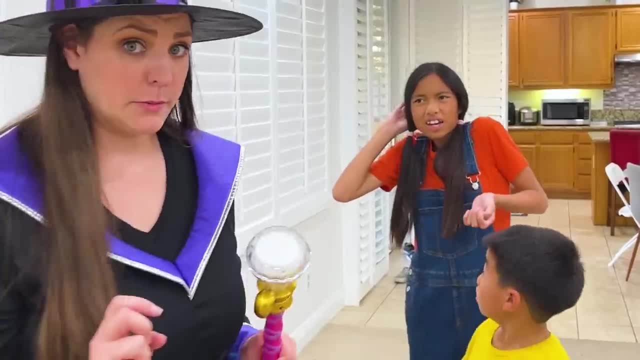 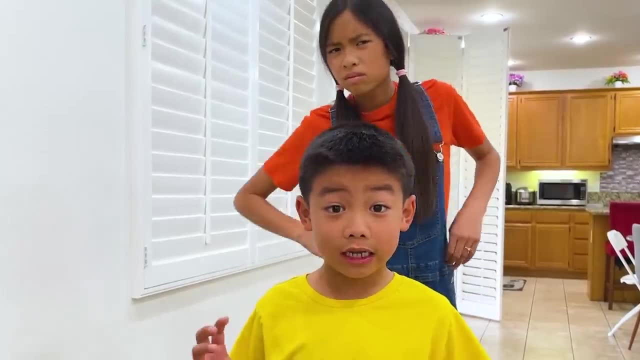 No running, Please No running. Ooh, Sorry, He don't take bath. There's no more paupet. Where can it be now? Hmm, Where? That's a good question. Excuse me, sir, This might sound strange, but have you seen a mummy? 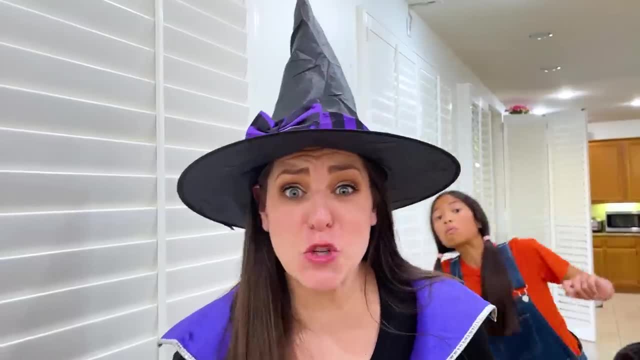 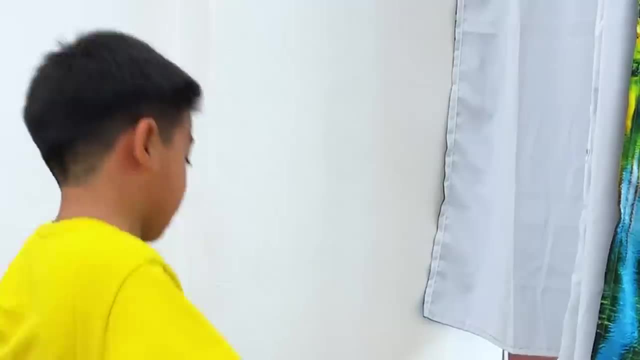 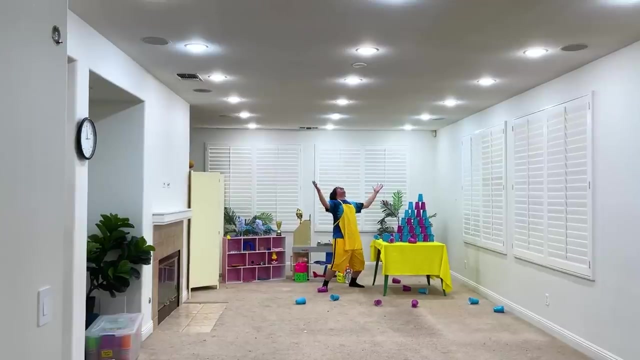 Yes, We went that way. That's back to the school. Hey kids, We have to get back to the school. Bye, No running, Okay. Bye No, Shaggy, No, Oh well, I guess I'll just start over. 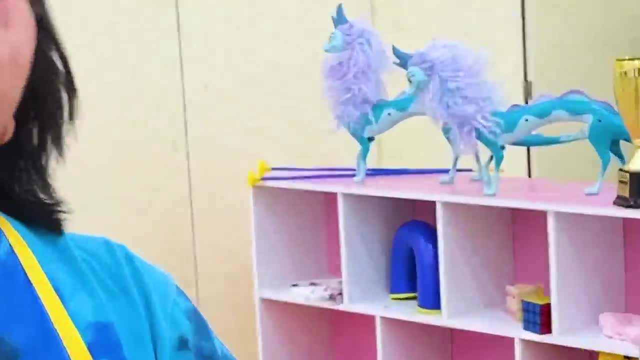 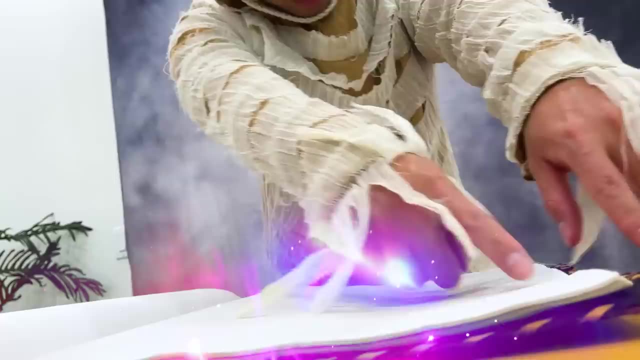 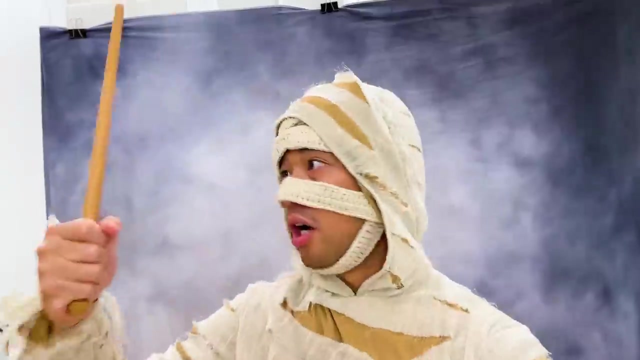 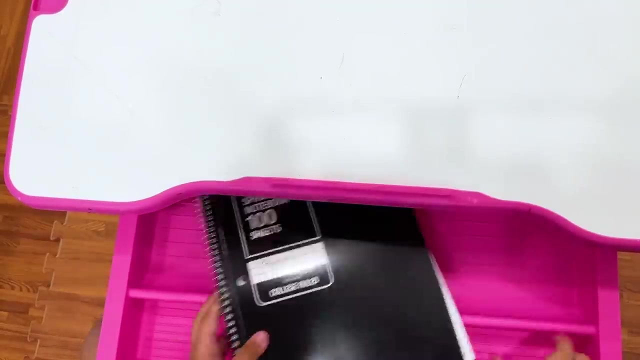 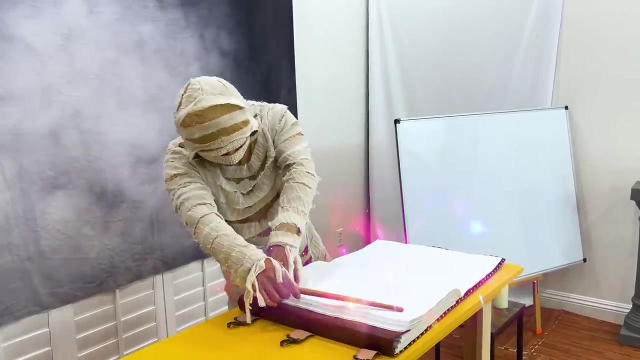 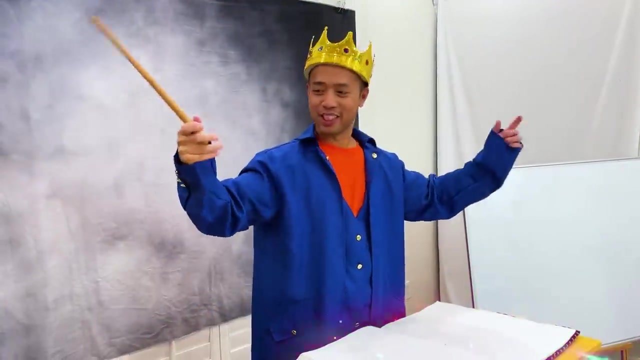 Oh no, Oh no, This was so fun. Do a substitute. Ah, Much better. Oh, He transformed. Oh. What else does this book have? Oh, The most powerful being, Oh, Yes, Most powerful being, Oh. 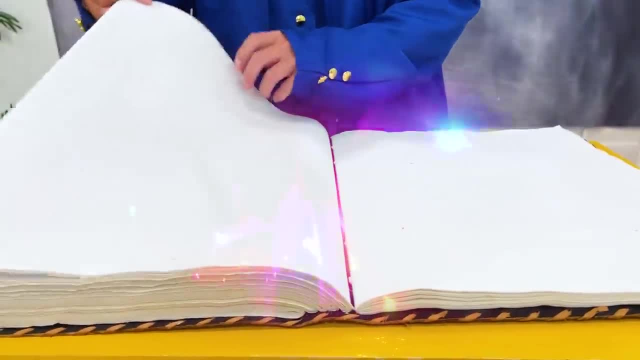 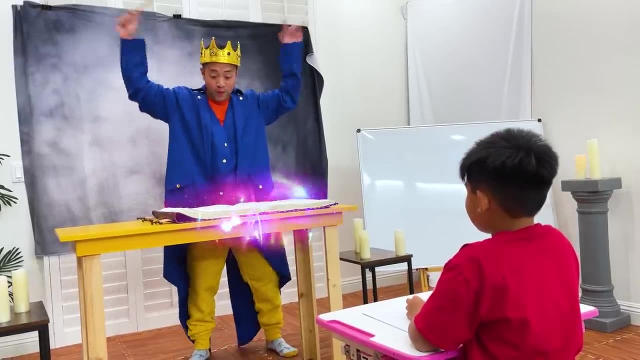 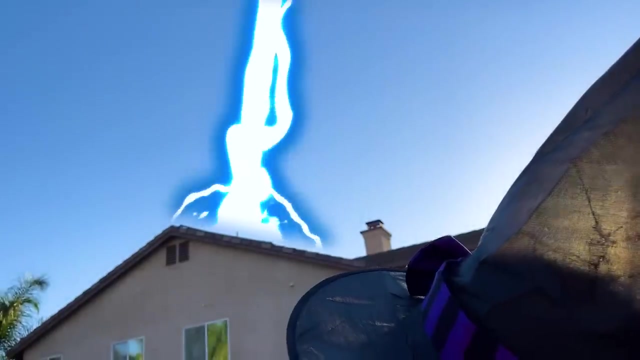